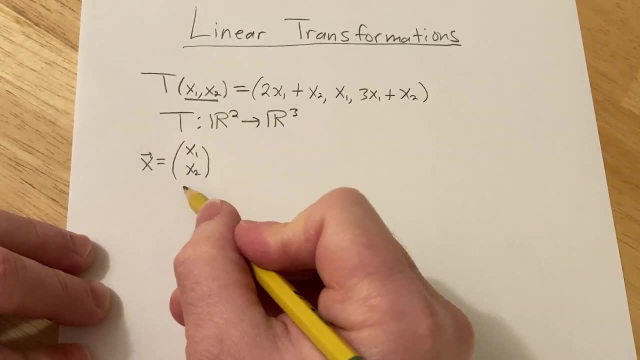 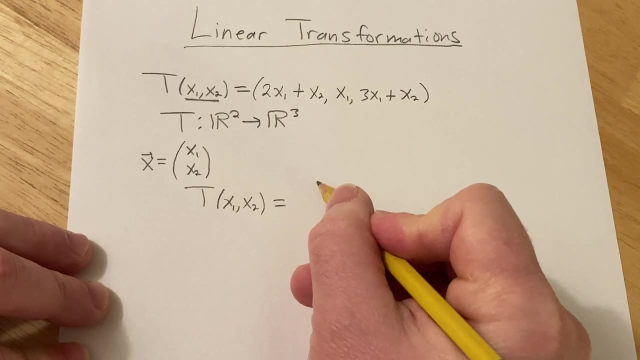 And then now I'm going to take t and write it a different way, just to show you, just to try to explain it. So I'm going to just keep this the same, but I'm going to write it like this. Watch this. So this is really 2x1, x2,. 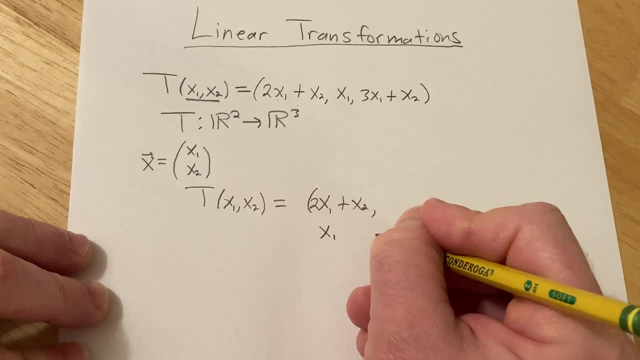 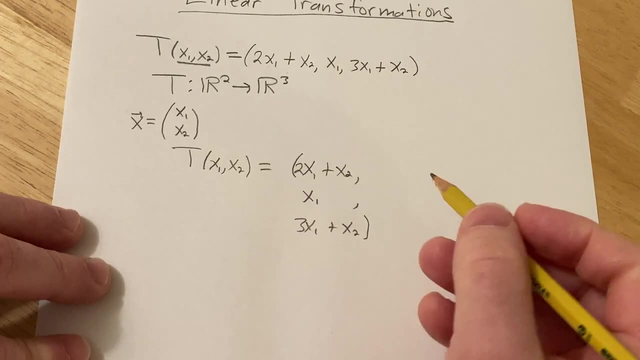 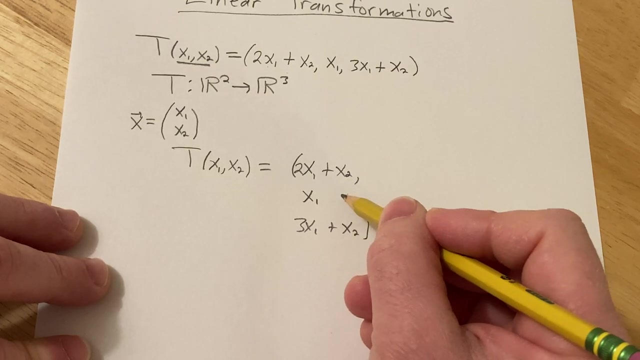 x1 and then 3x1 plus x2.. So you see it kind of looks like a matrix, right, And in fact it is. This is a matrix, So if you think about it very, very carefully, you could pretty much insert a zero here, okay, And then you can take this matrix here a. 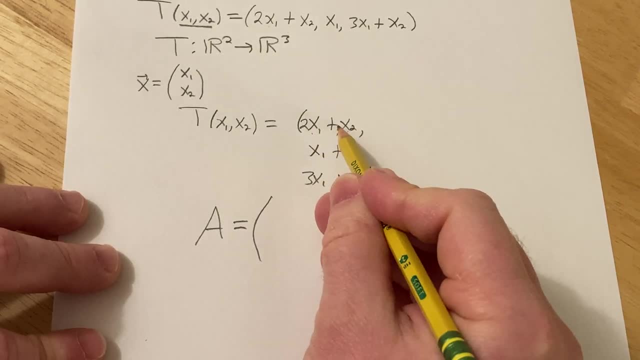 and so this matrix here would be 2, 1.. That's the coefficient there. You see that The coefficient is 1, and then 1, 0, and then 3, 1.. You see 1, 0,, 3, 1.. Just the coefficients. 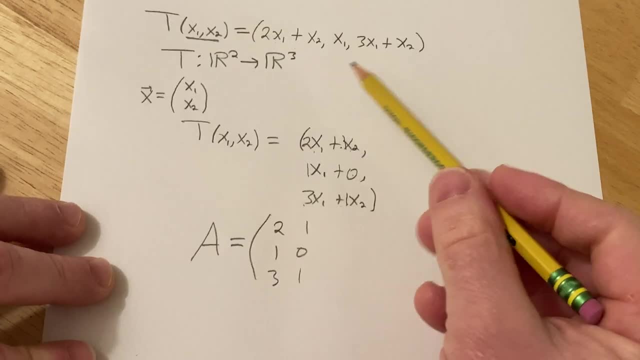 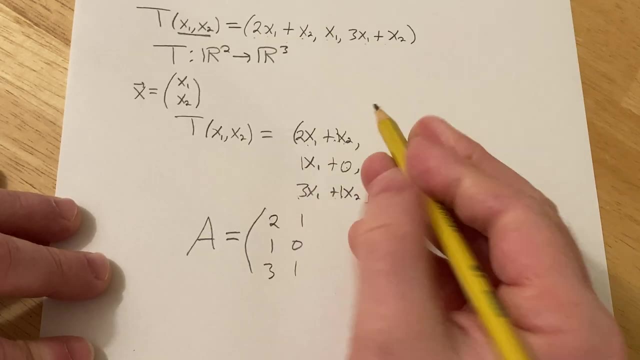 2, 1,, 1, 0,, 3, 1.. You can get it from here too, right, Look? 2, 1,, that's your first row. 1, 0,, that's your second row. 3, 1,, that's your third row. So what are we even doing? What is happening? 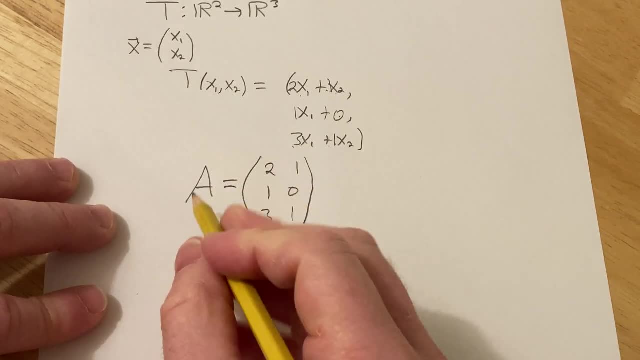 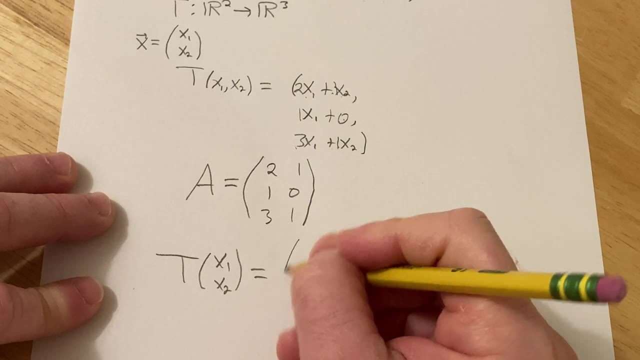 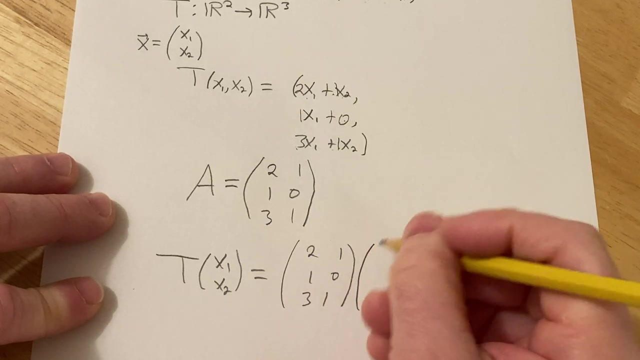 here. So now we can think about it a different way. So now I'm going to use the vector notation. So t of x1, x2 is actually equal to 2, 1, 1, 0, 3, 1 times x1, x2.. 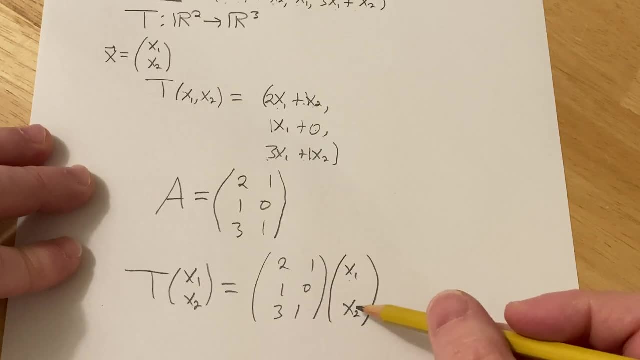 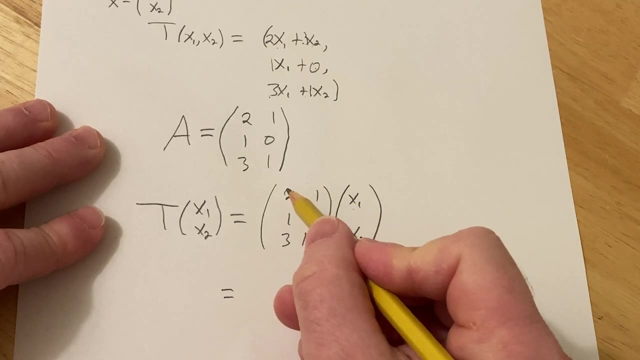 It's actually the same thing, right? The claim is that this is the same thing as what we started with, And it is right It actually is. If you multiply this out, this is a 1,, 2, 3 by 2 matrix. 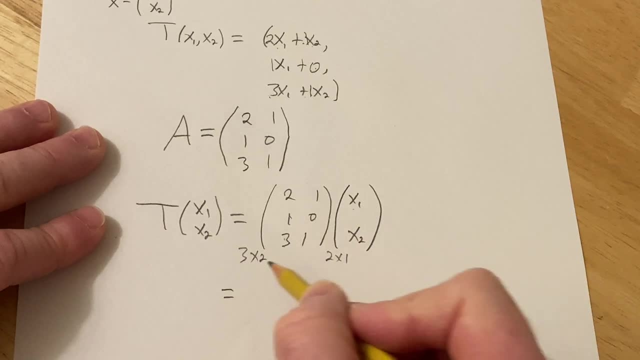 this is a 2 by 1 matrix or just a column vector. So when you multiply this, you're going to get a 3 by 1 matrix. So we'll get 3 rows and 1 column. So let's do it. Let's multiply it 2 times x1. 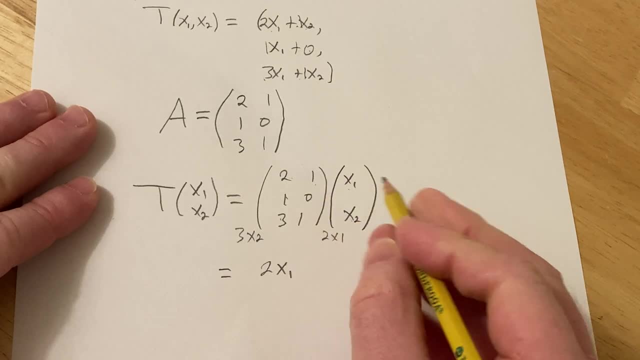 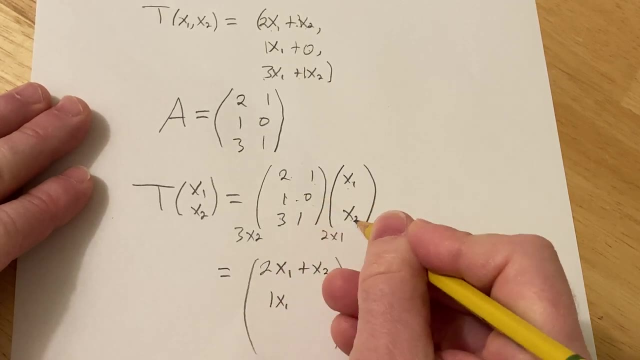 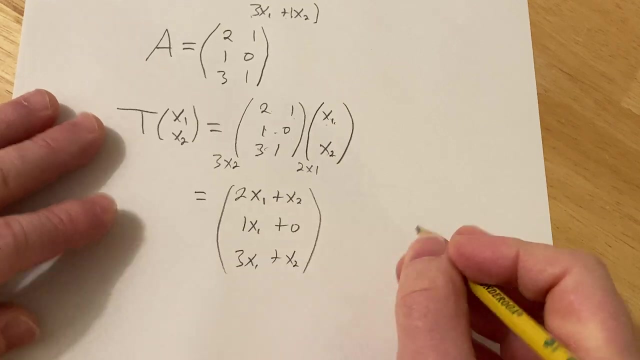 is 2 times x1.. 1 times x2 is 1 times x2.. So, plus that, 1 times x1, 0 times x2.. 3 times x1, 1 times x2.. So you see, this is exactly what we have at the beginning. So this is the same thing. 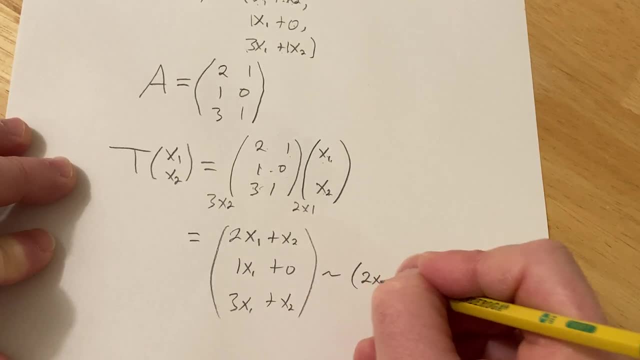 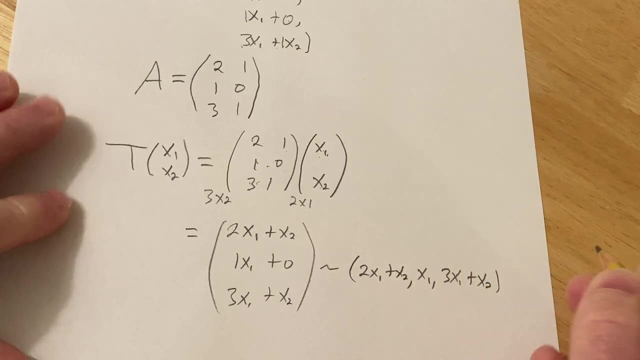 People write it. Instead, they write it like this: They write it at 2x1 plus x2, x1, 3x1 plus x2.. So that's why it's the same And you can use shorthand for this right You. 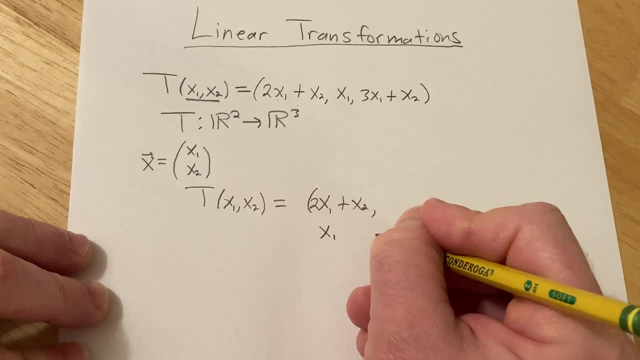 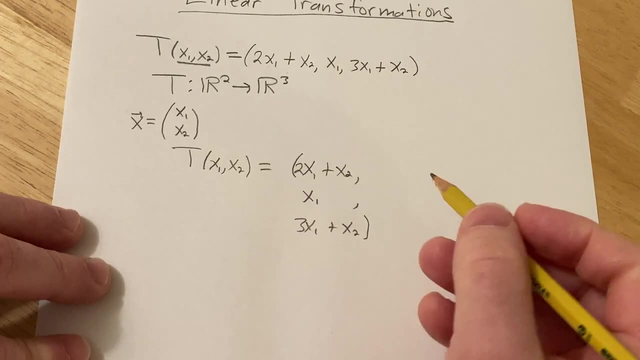 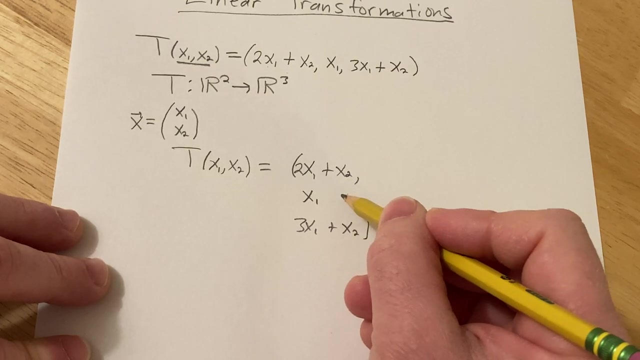 x1 and then 3x1 plus x2.. So you see it kind of looks like a matrix, right, And in fact it is. This is a matrix, So if you think about it very, very carefully, you could pretty much insert a zero here, okay, And then you can take this matrix here a. 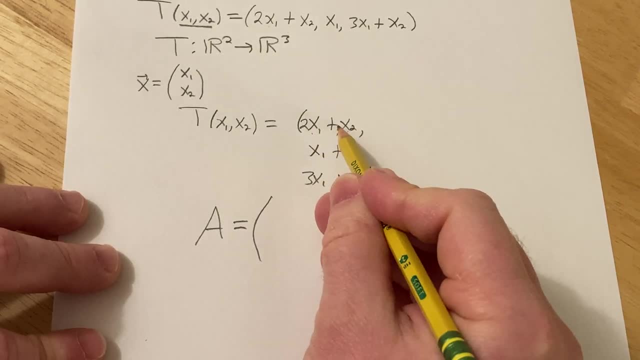 and so this matrix here would be 2, 1.. That's the coefficient there. You see that The coefficient is 1, and then 1, 0, and then 3, 1.. You see 1, 0,, 3, 1.. Just the coefficients. 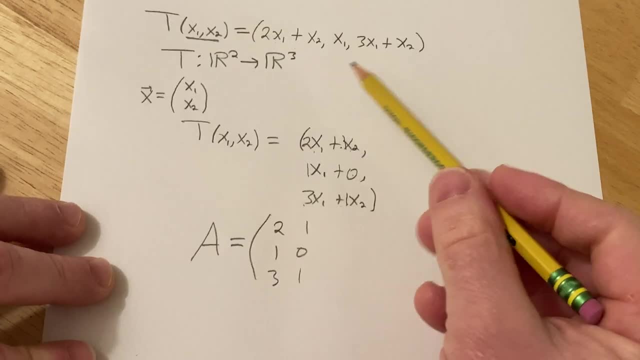 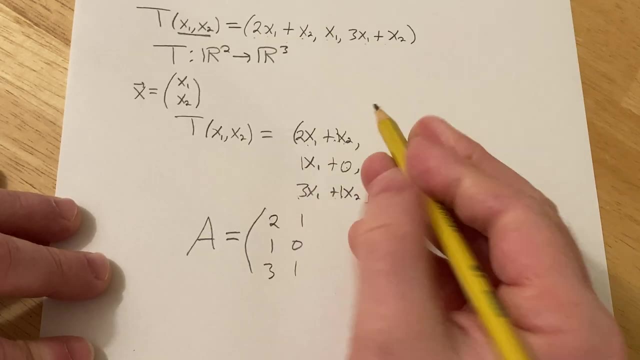 2, 1,, 1, 0,, 3, 1.. You can get it from here too, right, Look? 2, 1,, that's your first row. 1, 0,, that's your second row. 3, 1,, that's your third row. So what are we even doing? What is happening? 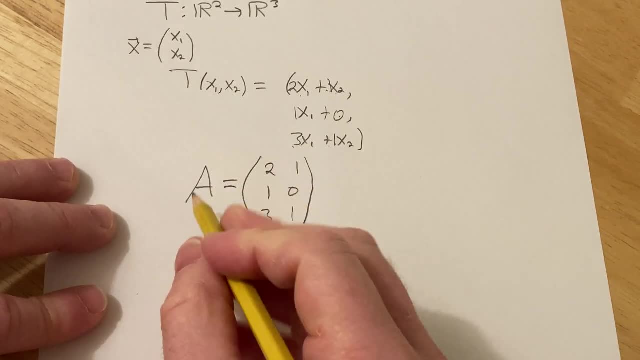 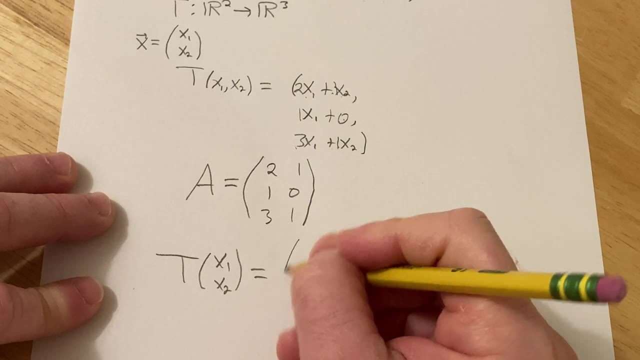 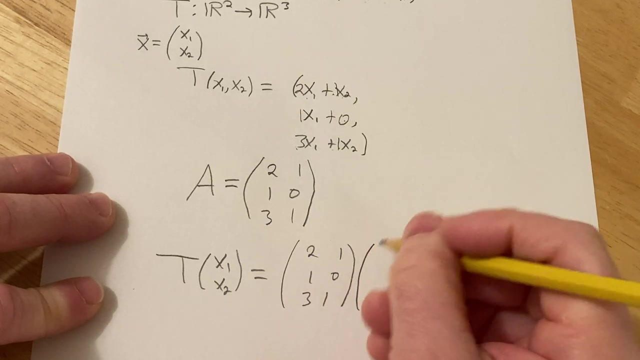 here. So now we can think about it a different way. So now I'm going to use the vector notation. So t of x1, x2 is actually equal to 2, 1, 1, 0, 3, 1 times x1, x2.. 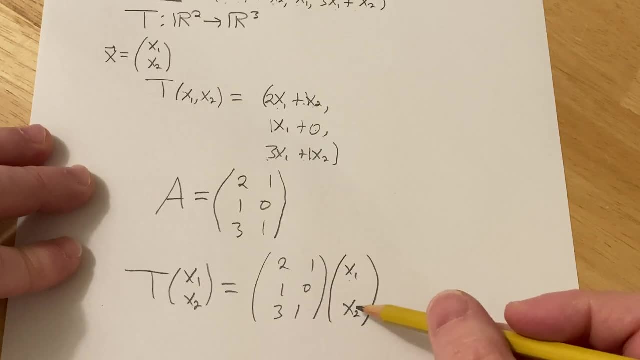 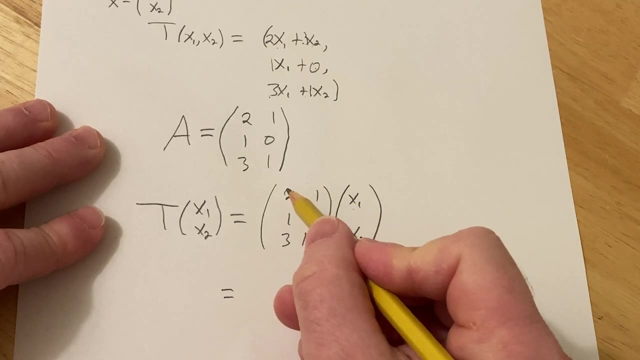 It's actually the same thing, right? The claim is that this is the same thing as what we started with, And it is right It actually is. If you multiply this out, this is a 1,, 2, 3 by 2 matrix. 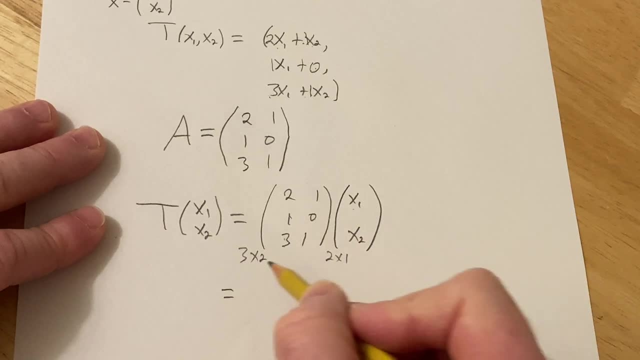 this is a 2 by 1 matrix or just a column vector. So when you multiply this, you're going to get a 3 by 1 matrix. So we'll get 3 rows and 1 column. So let's do it. Let's multiply it 2 times x1. 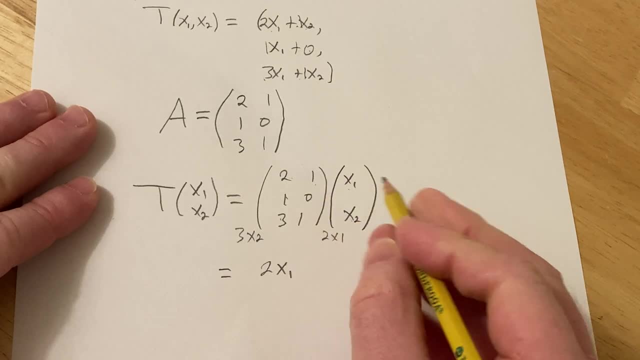 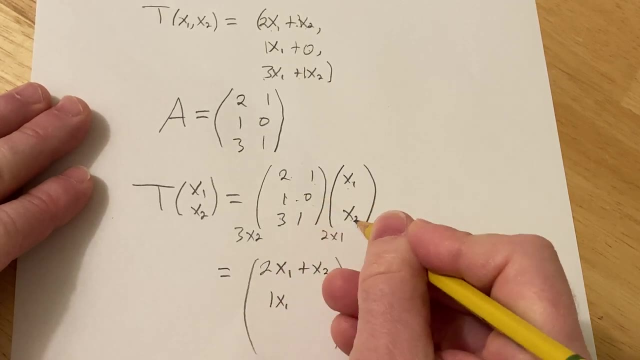 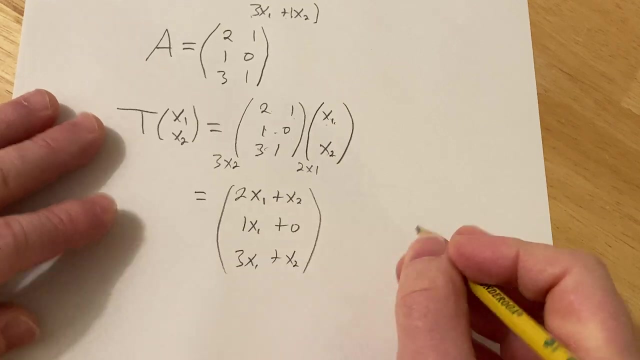 is 2 times x1.. 1 times x2 is 1 times x2.. So, plus that, 1 times x1, 0 times x2.. 3 times x1, 1 times x2.. So you see, this is exactly what we have at the beginning. So this is the same thing. 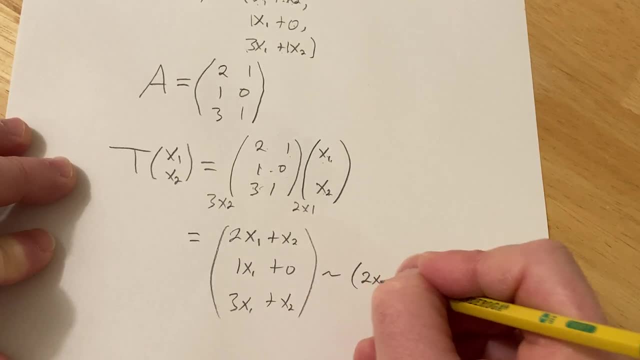 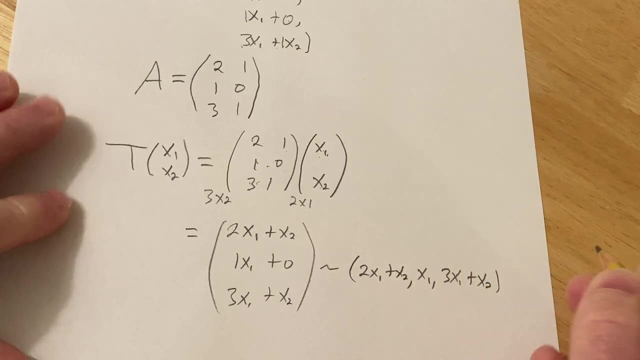 People write it. Instead, they write it like this: They write it at 2x1 plus x2, x1, 3x1 plus x2.. So that's why it's the same And you can use shorthand for this right You.